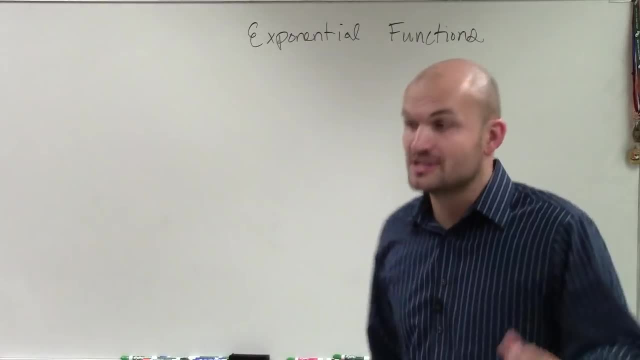 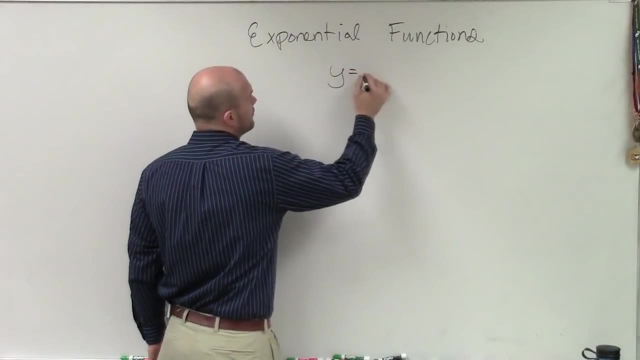 but what exactly does the graph look like? It doesn't take much, ladies and gentlemen, for us to be able to plot in a graph, but let me go and show you the general form of an exponential. So remember, exponential. we have y equals a to the x right, And I'm 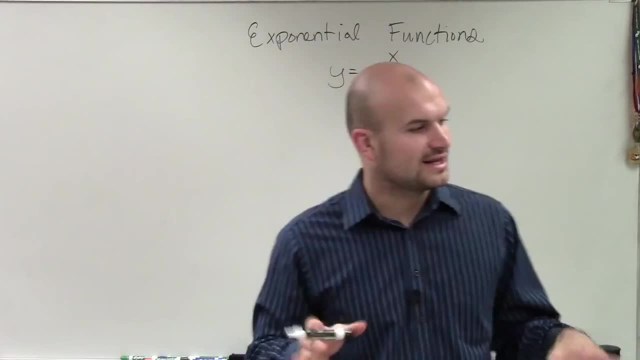 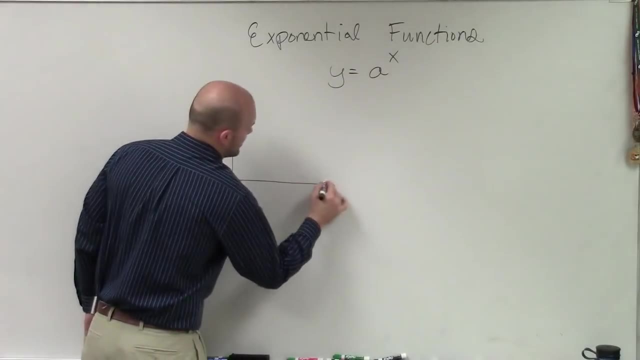 just going to show you the basic format of what exactly the graph is going to look like and some kind of special features. Then I'll show you how to graph one the long way, because you always want to look at the long way. so then you can always know you know what if. 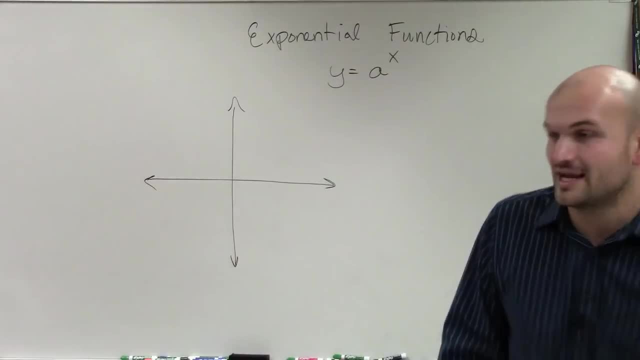 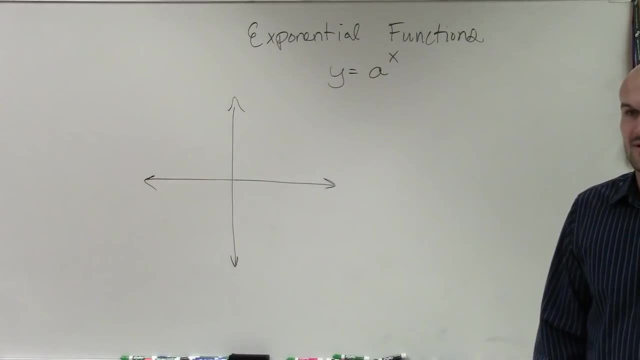 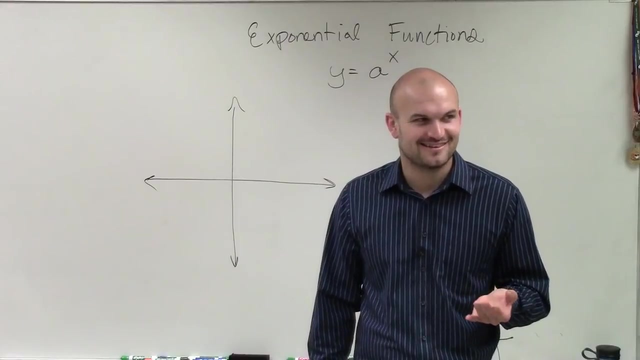 I don't have a graphing calculator and I need to know how to graph this, and I forgot how the transformations work. I know I can always, always- always- use a gable and a taff. What do you think that is A table and a graph? You can always use a table of values. 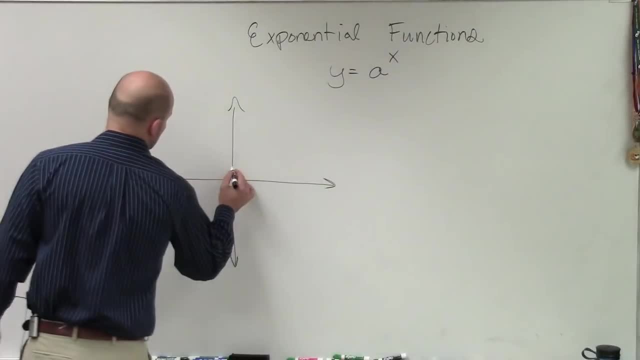 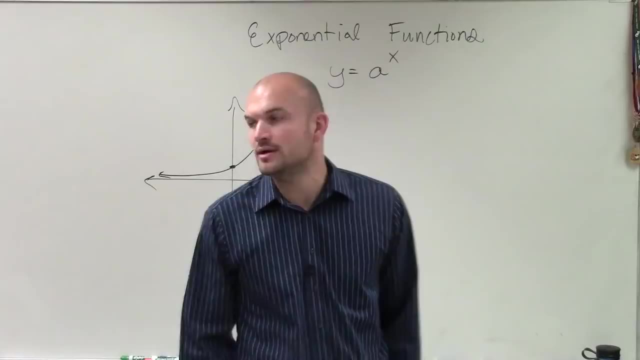 and a graph. But anyways, let's go ahead and take a look at what this function is going to look like and I'll show you why That is going to be. the general form of y equals a to the x. all right, So there's a couple things I want you guys to understand. First, 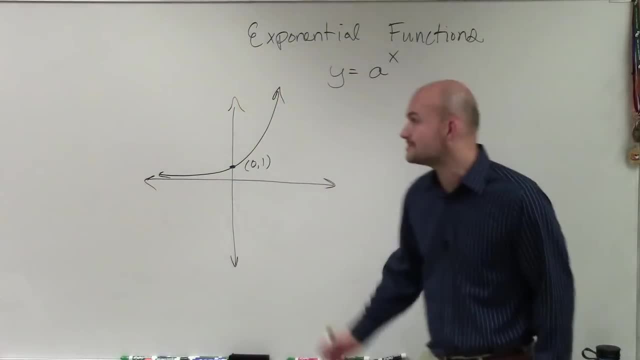 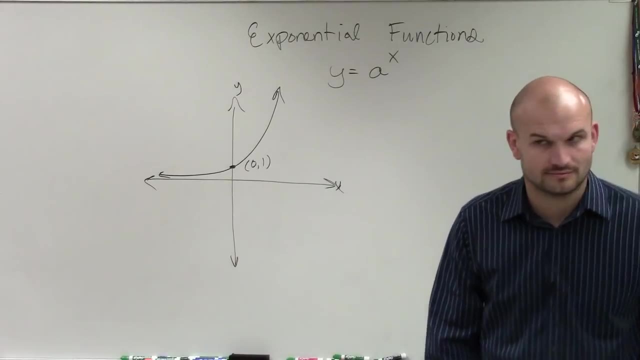 of all, it has a y intercept. right, Here's your y axis, x axis, And then you have the x. It has a y intercept of 0 comma 1, all right. Also, you guys can see that, this graph. 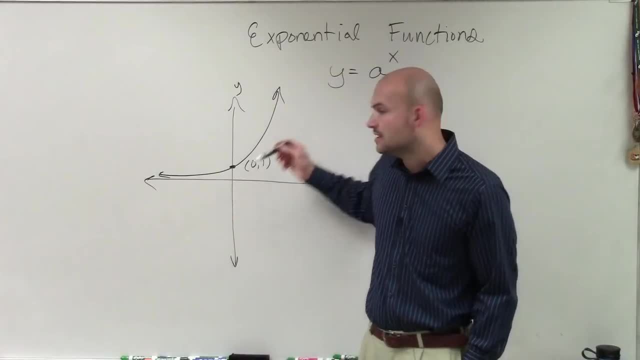 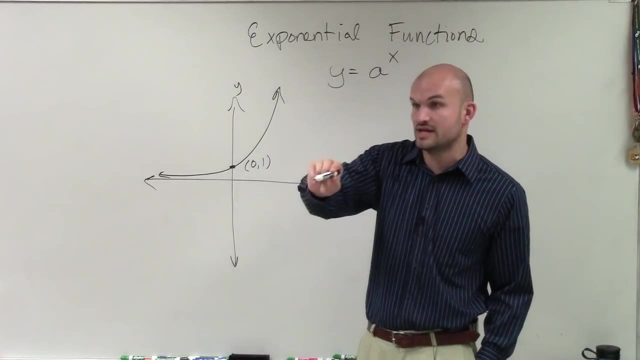 it looks like it keeps on approaching, And we're going to talk more about asymptotes later, because we didn't really get to touch them in rational function. Yes, Do you need another seat? Oh, that was fun. OK, So you guys can see that it's approaching 0, but 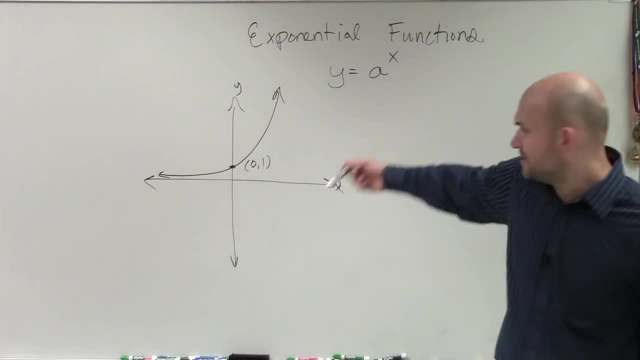 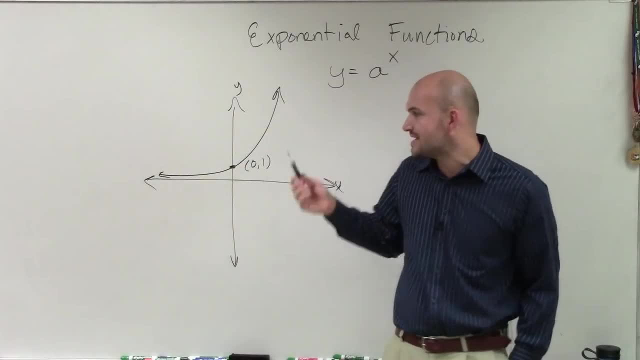 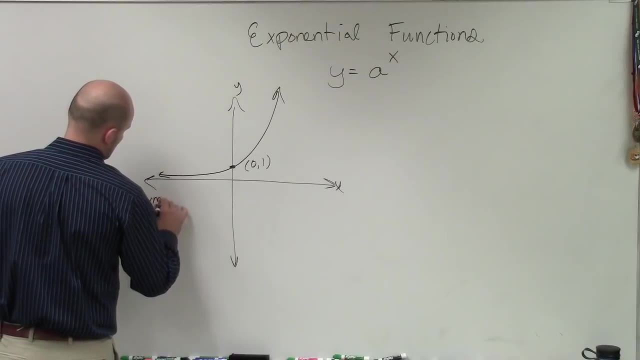 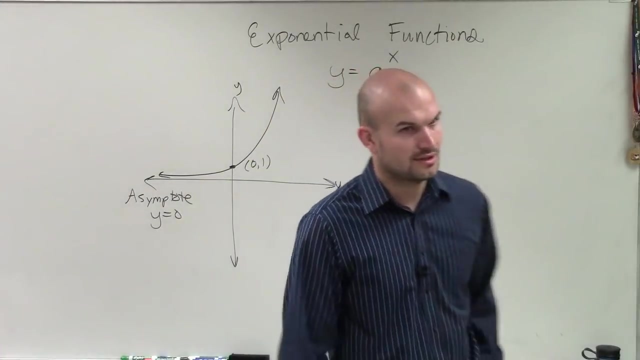 doesn't have any negative values to it, right? So what it is is we say it's approaching our vertical line of y equals 0. So you can say it has an asymptote of y equal 0. What that means is it's going to keep on. the graph is going to keep on approaching those y equals. 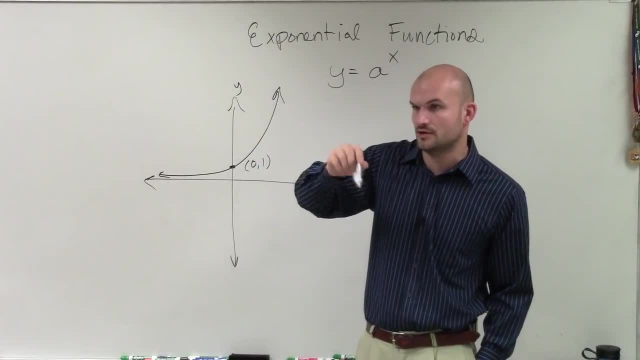 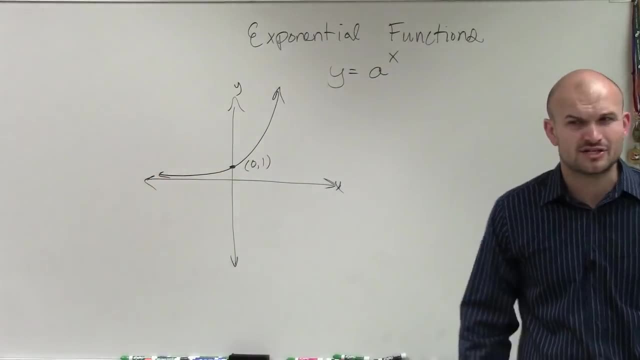 Yes, Do you need another seat? Oh, that was fun. OK, So you guys can see that it's approaching 0, but it actually never crosses This graph. that actually doesn't go. It doesn't look like it doesn't right now in my form of value. 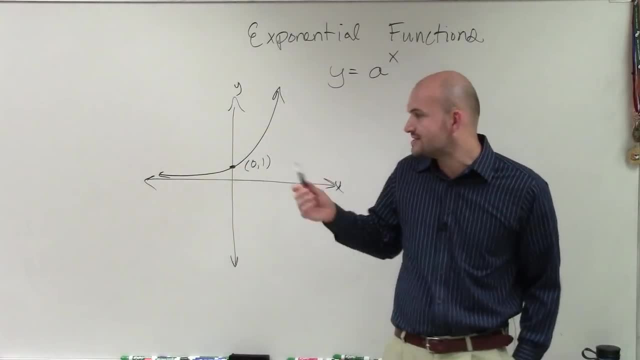 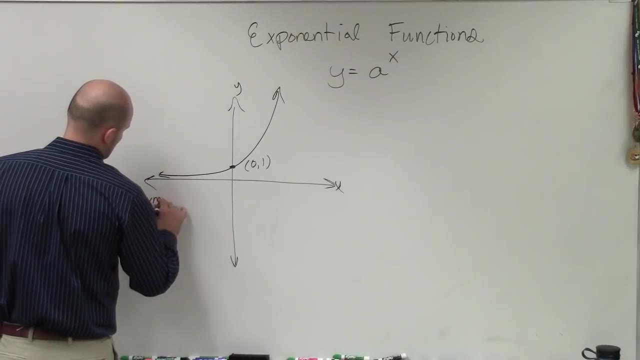 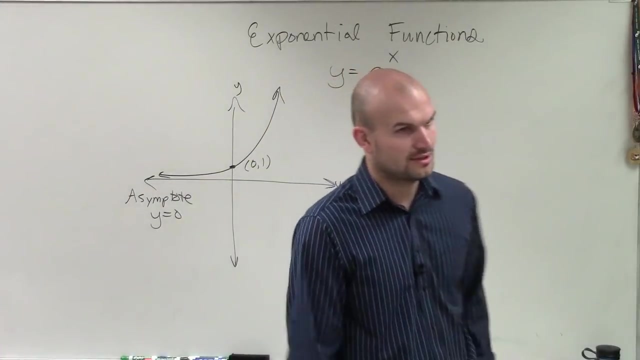 it doesn't have any negative values to it, right? So what it is is we say it's approaching our vertical line of y equals 0. So you can say it has an asymptote of y equals 0. What that means is it's going to keep on. 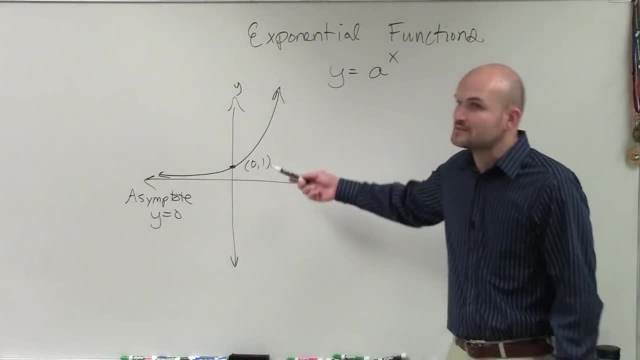 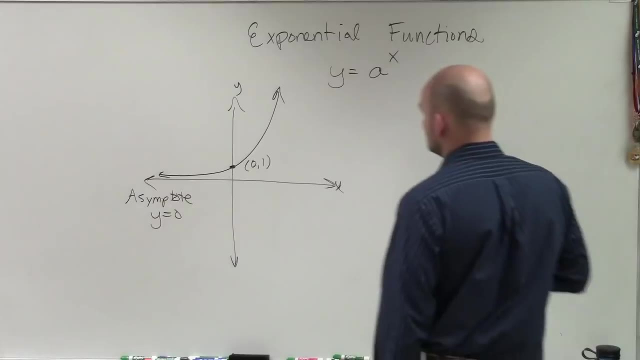 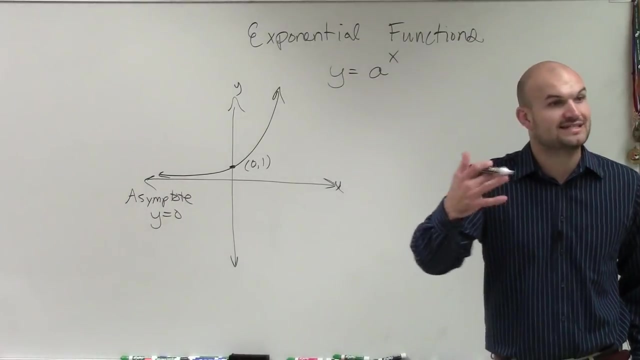 the graph is going to keep on approaching those y equals 0.. And guess what? It's not going to go below it unless we start ending up having some transformations for the graph. And then, obviously, where the exponential is mostly used in our language is we say something grows or decays. 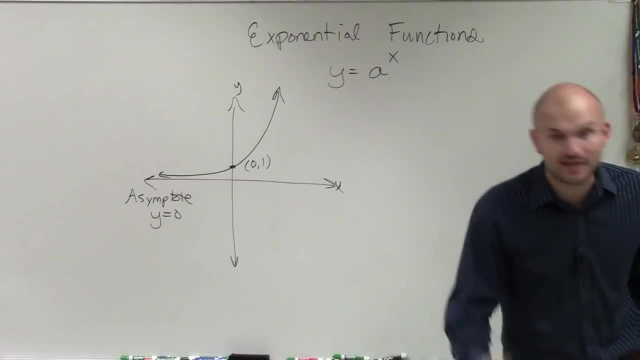 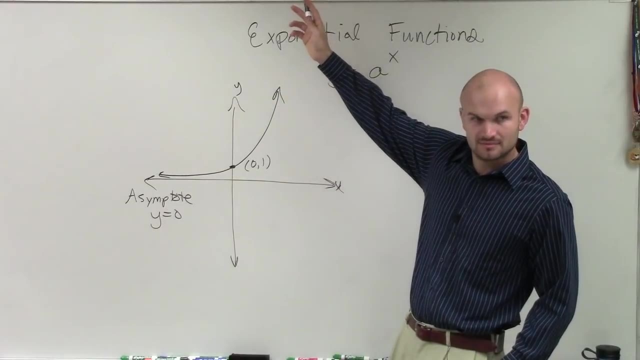 exponentially right. The growth of the population is exponential growth Because you can see as something grows. this just keeps on getting steeper and steeper and steeper, right. OK, So we'll talk a little bit more about exponential growth. 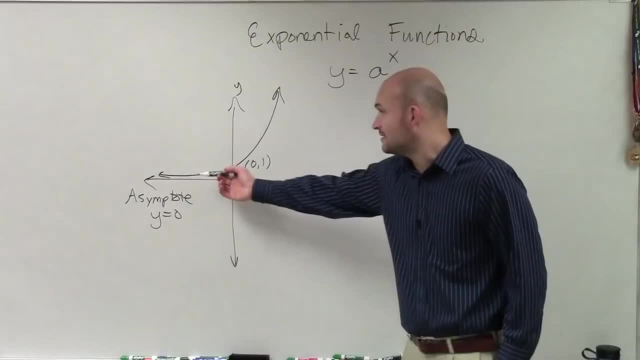 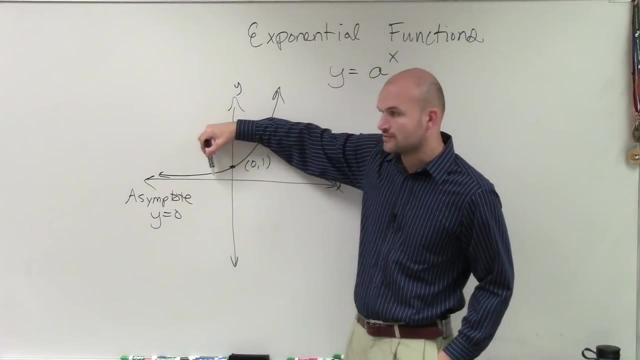 and decay, but a lot of times when we use that, you can see this graph. you know, if you start here, that growth is very small. Yes, Very, very small growth. But then once you kind of hit a threshold, 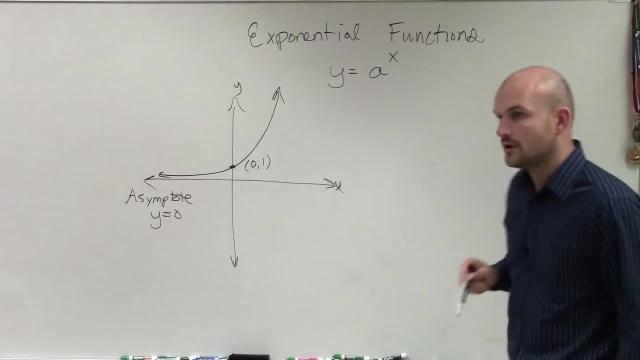 this growth just keeps on getting bigger and bigger. All right, So let's go and take a look at an example. And again, this doesn't matter if you have multiple transformations or just a basic graph, But let me just kind of give you an example of x equals. 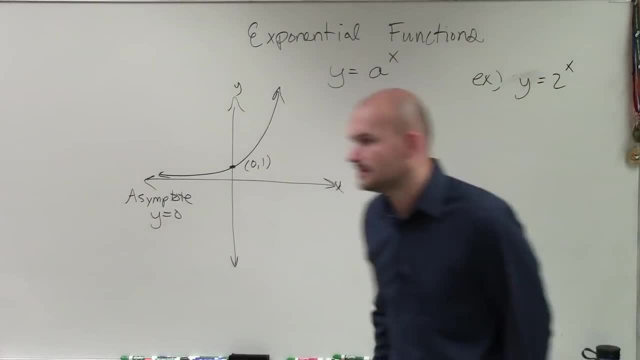 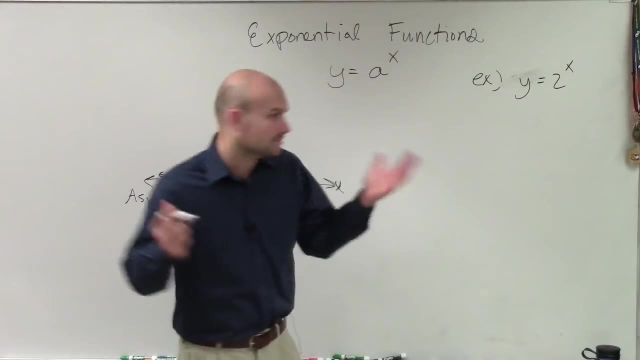 let's graph: y equals 2 to the x. All right, So I'm just going to give you guys a basic way to do this. This is a basic way to remember how to graph If you, ladies and gentlemen, need to know how to graph. 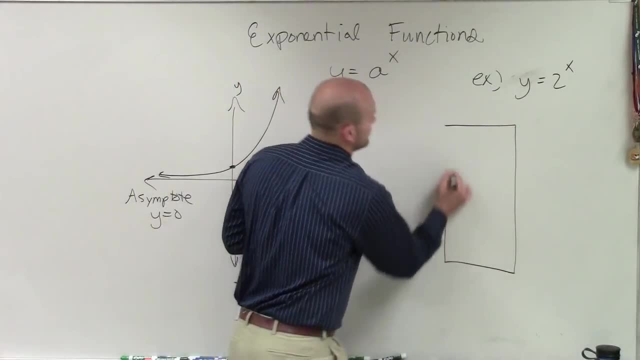 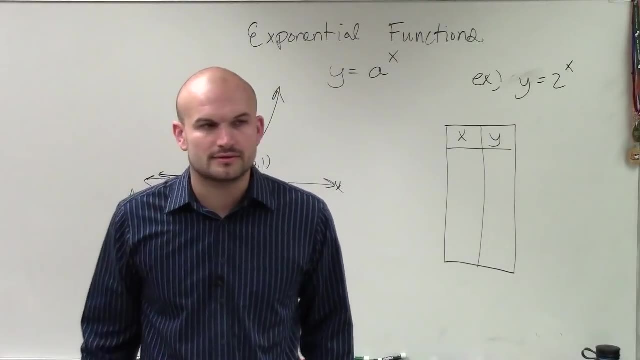 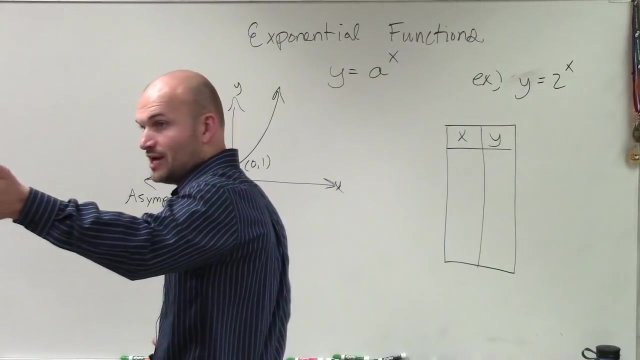 you can always go back to a table of values. Always, When completing a table of values, we just have our x and our y values, And then we're just going to choose which values we want to pick. So what do? you got a value. you want to try. 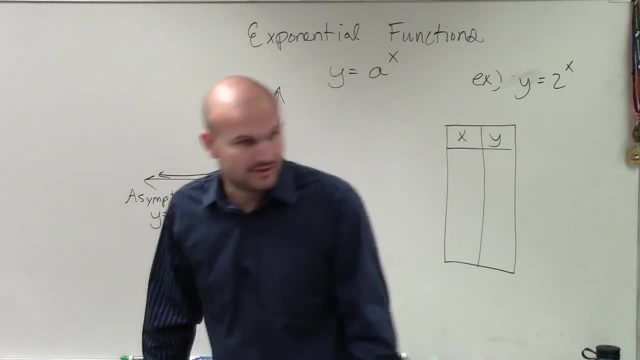 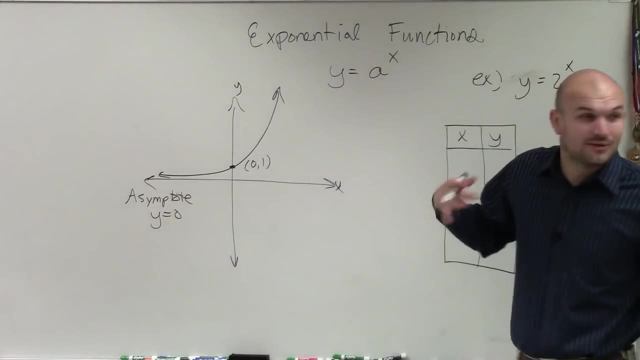 2. Adar, do you got a value 1. OK, 1. Brandi, you got a value 30.. 3. OK, Well, yeah, 3,, 2,, 1.. You guys are very good. 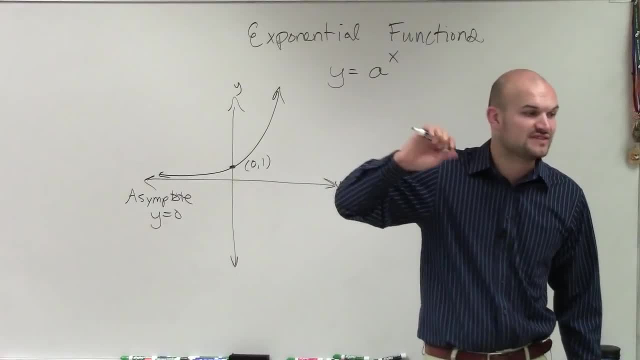 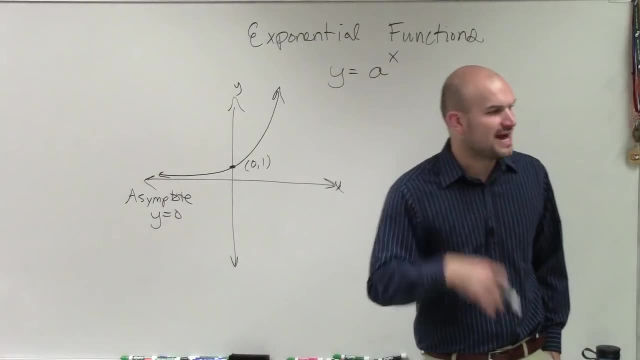 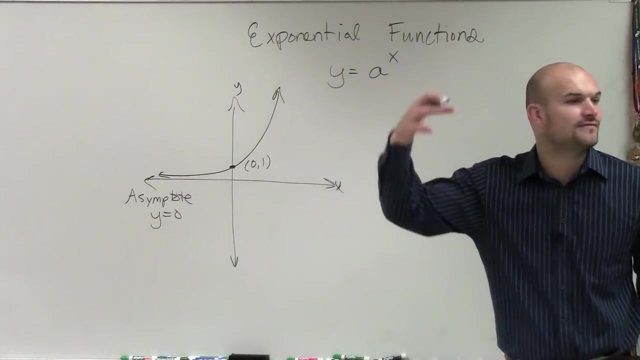 0. And guess what? It's not going to go below it, unless we ended up having some transformations for the graph. And then, obviously, where the exponential is mostly used in our language is we say something grows or decays exponentially, right, The growth of the population is exponential growth because you can see as something grows. 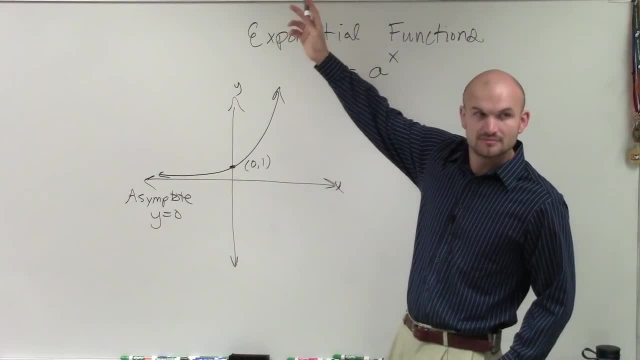 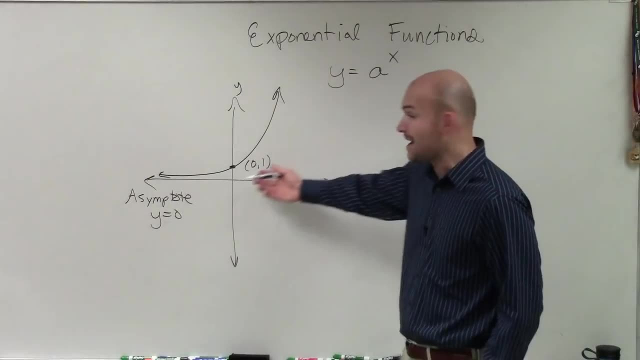 this just keeps on getting steeper and steeper and steeper, right. So we'll talk a little bit more about exponential growth and decay, but a lot of times we'll use that. If you look at this graph, you know, if you start here, that growth is very small. yes, 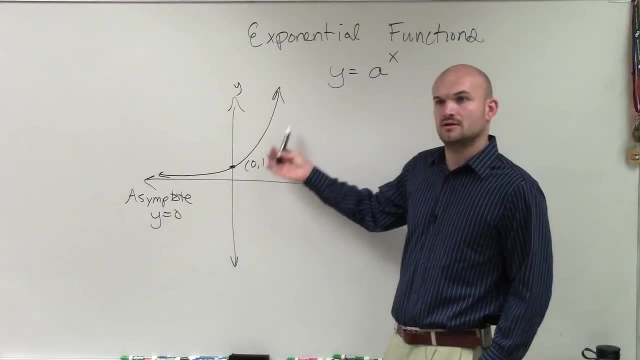 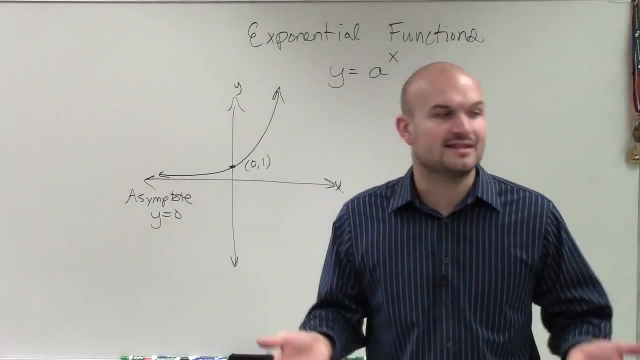 Very, very small growth, But then, once you kind of hit a threshold, this growth just keeps on getting bigger and bigger. all right, So let's go and take a look at an example. And again, this doesn't matter if you have multiple transformations or just a basic graph. 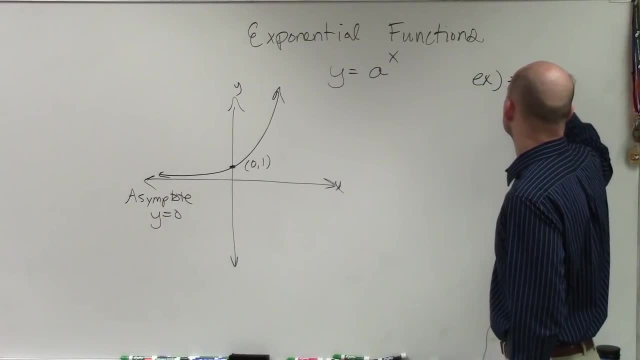 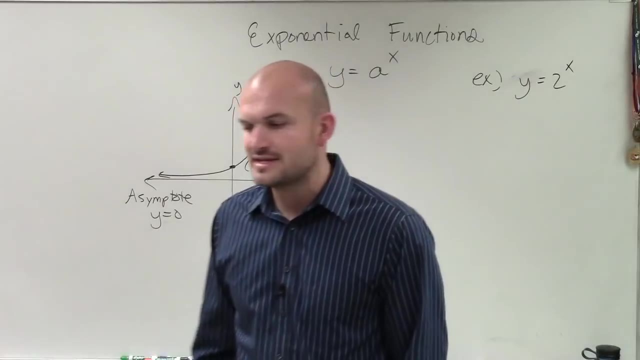 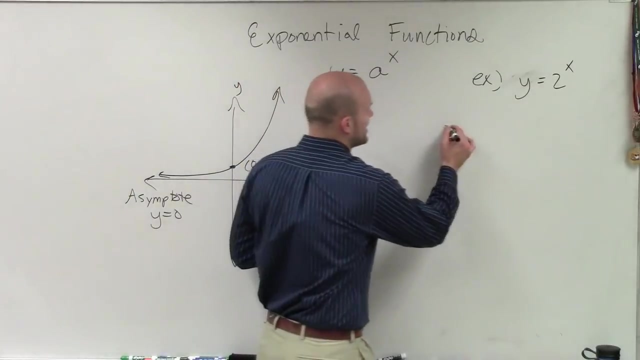 but let me just kind of give you an example of x equals- let's graph: y equals 2 to the x. all right, So I'm just going to give you guys a basic way to remember how to graph. If you, ladies and gentlemen, need to know how to graph, you can always go back to a 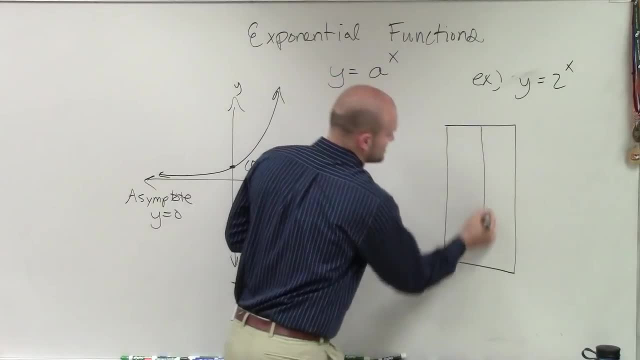 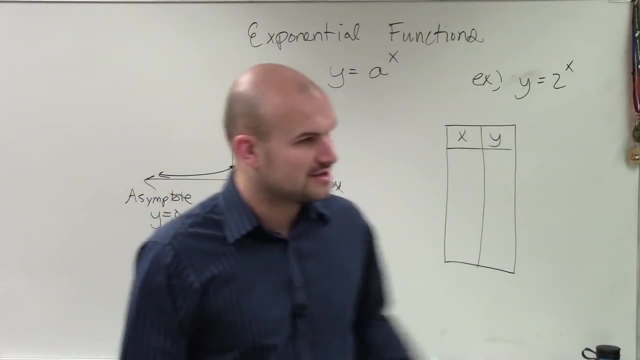 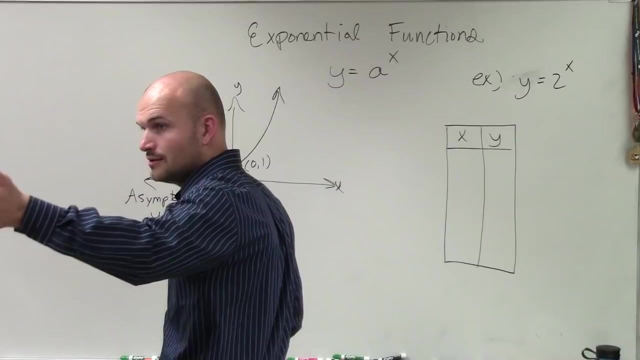 table of values. always, When completing a table of values, we just have our x and our y values and then we're just going to choose which values we want to pick. So what do you? got a value. you want to try 2.. 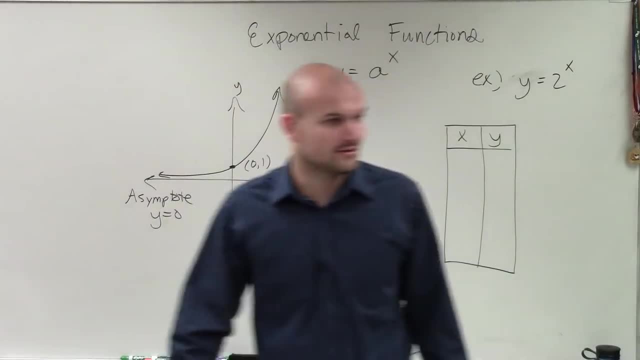 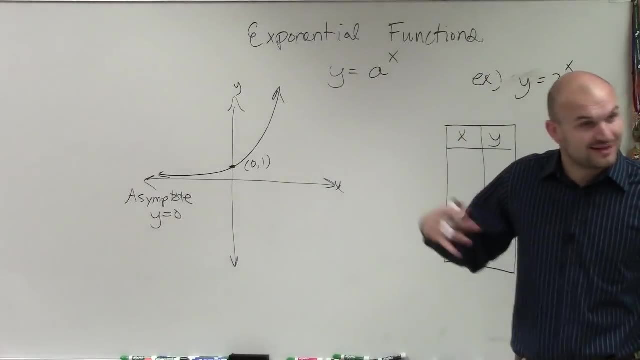 2. Adar, do you got a value 1. 1. 1. OK, Brandy, you got a value 30. 3. OK, Well, yeah, 3,, 2,, 1.. 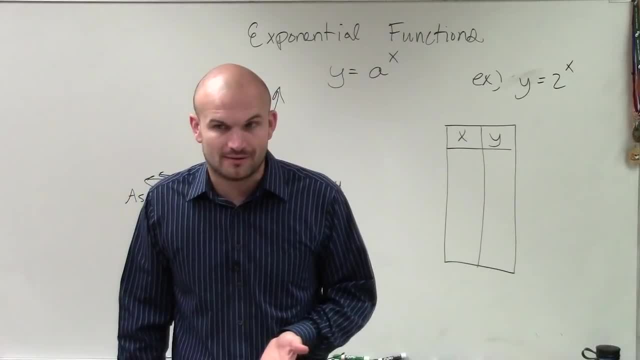 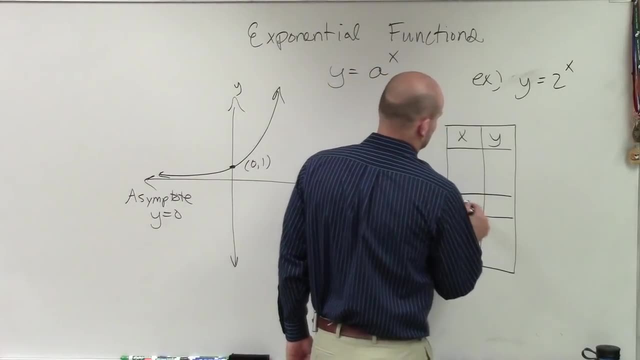 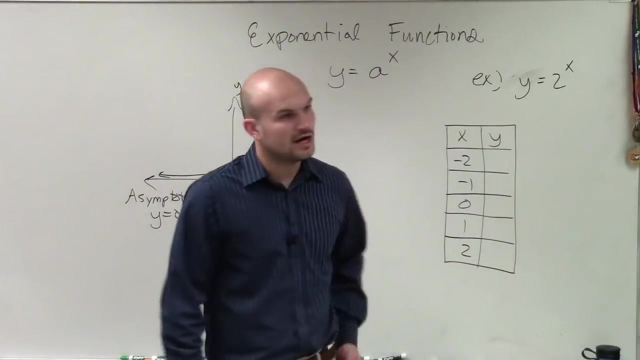 You guys are very good. I would also recommend trying some negative values as well. all right, And also 0 is always a really good one to use. Now, to keep this video a little bit short, I'm only going to use the values of 1,, 2,. 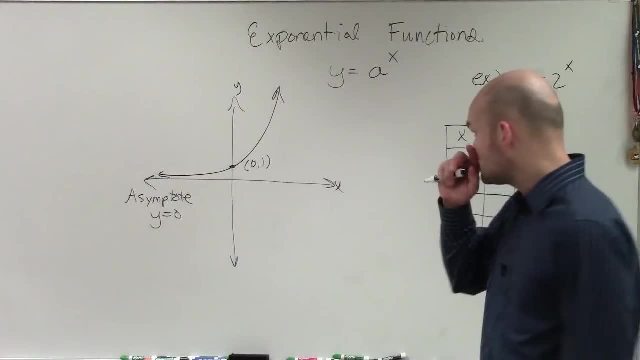 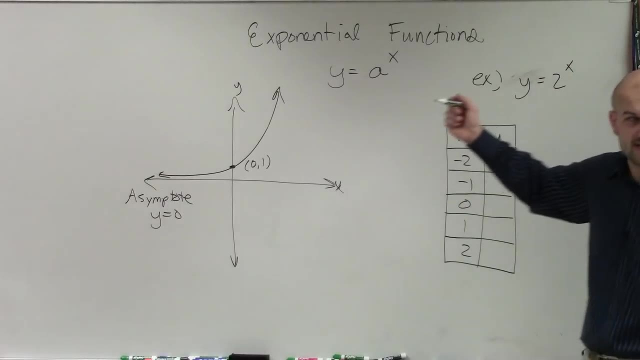 negative 1, negative 2, and 0.. All right, So, if you guys remember, what do we do with these table values? How do we create a table of values? If I have y equals 2 to the x? we do what with our values of x. 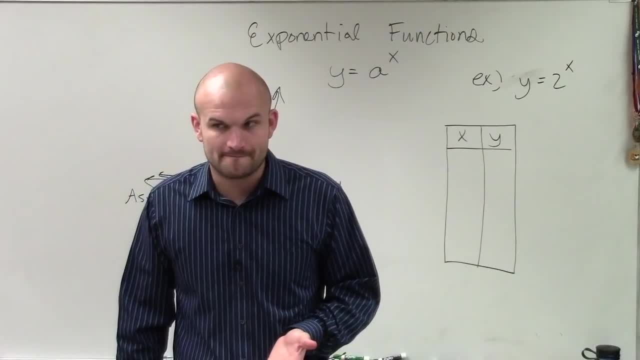 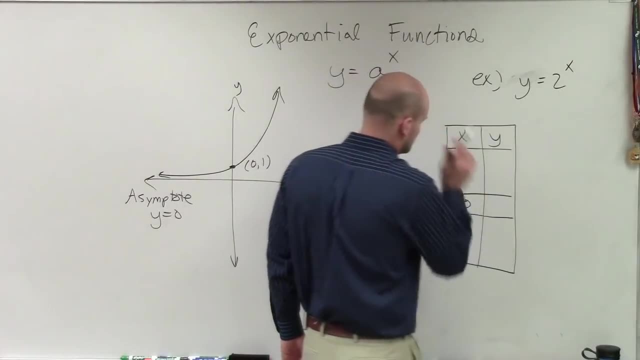 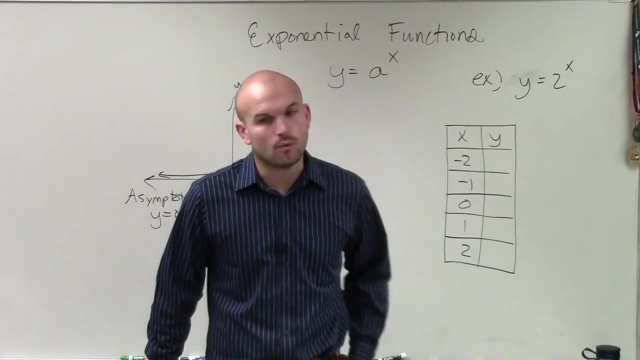 I would also recommend trying some negative values as well. All right, And also 0 is always a really good one to use. Now, to keep this video a little bit short, I'm only going to use the values of 1,, 2, negative 1,. 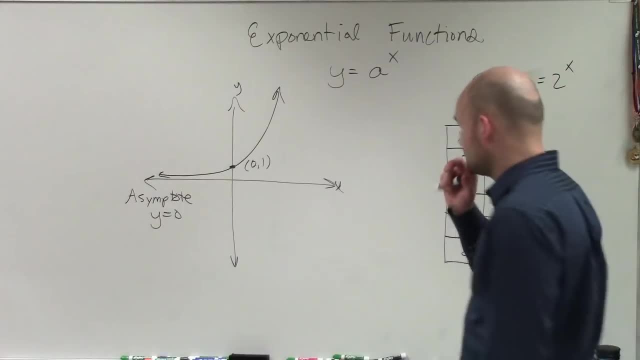 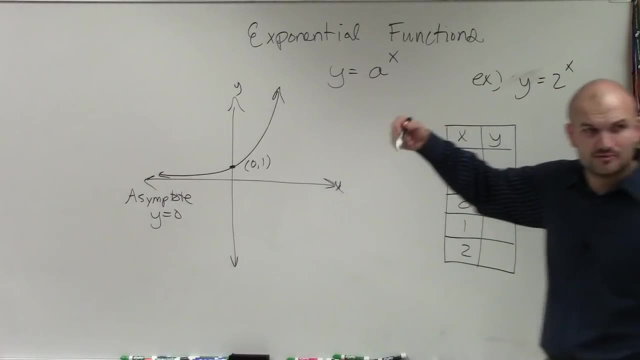 negative, 2, and 0.. All right, So, if you guys remember, what do we do with these table values? How do we create a table of values? If I have y equals 2 to the x, we do what with our values of x. 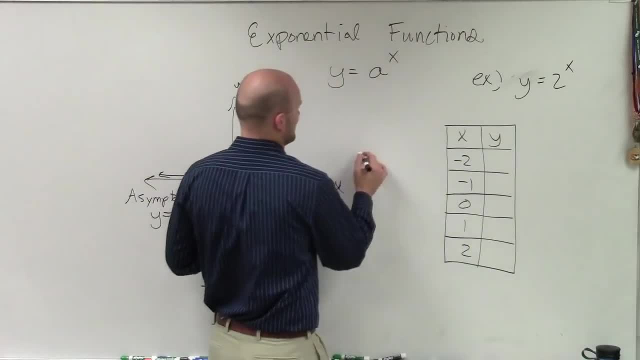 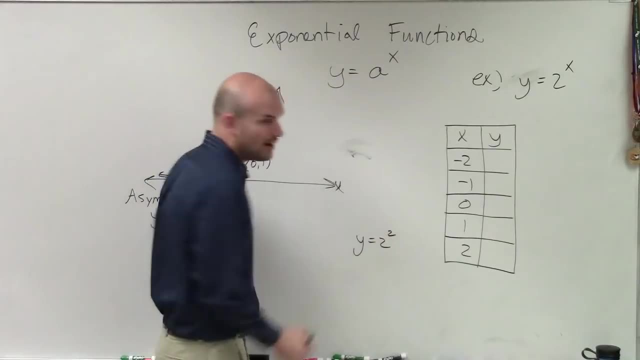 Plug them in. Then you find the value of y Right. OK, So let's start with the positive so we can remember what it looks like. So I'd have: y equals 2 squared. Well, we know, 2 squared, right. 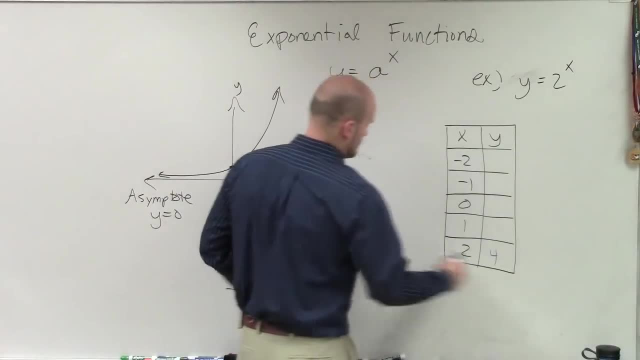 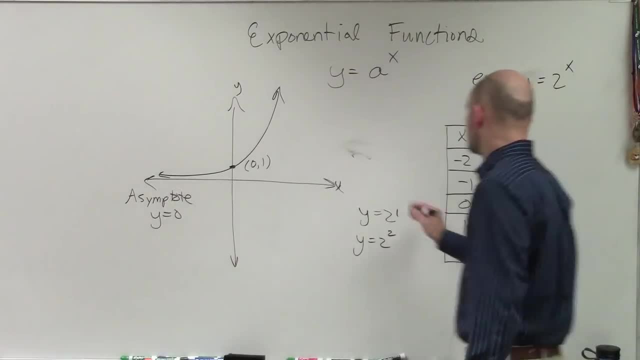 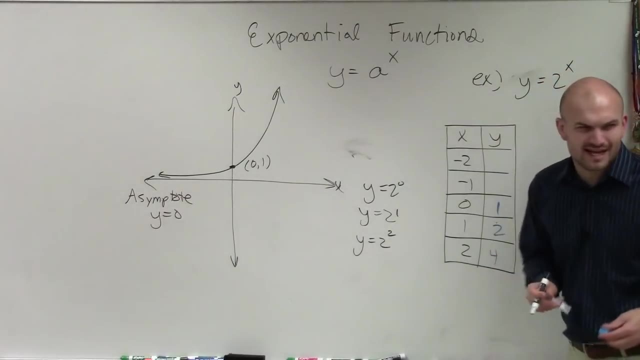 So then we have: y equals 2 to the 0 power 1. 1.. Very good, That's always going to be 1, right, And what I want you guys to understand. some of you might say: well, what happens if my base is 10?? 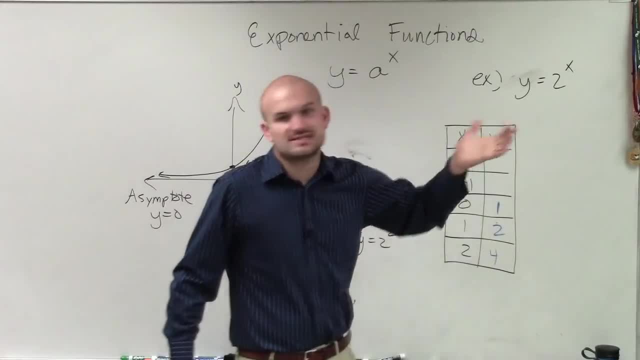 Because we're going to use a lot of different bases, right? What happens if my base is 10?? What happens if my base is 8?? What happens if my base is 1 half? You know how is that going to change the graph? 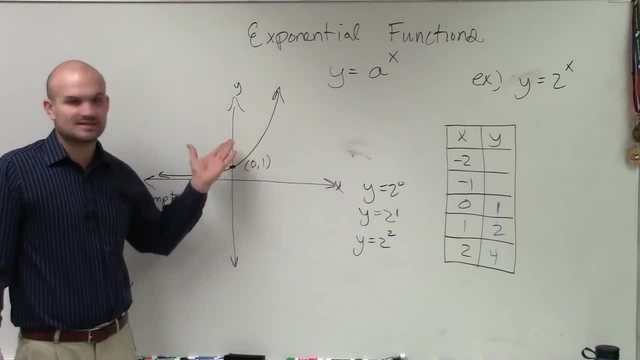 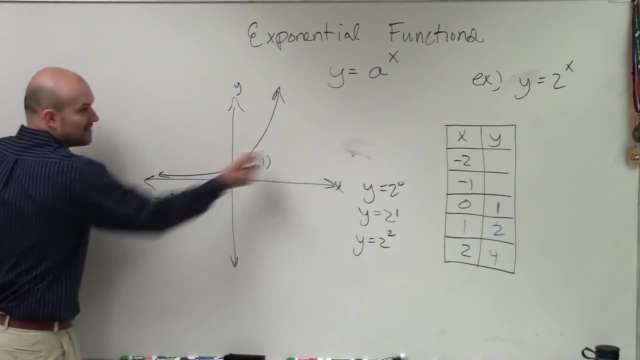 Well, one thing it is going to affect: 2. how the graph increase to where it's at. But you guys notice, does it matter what the base is when I raise it to the 0 power? No, So all of my exponential graphs, unless we have a transformation. 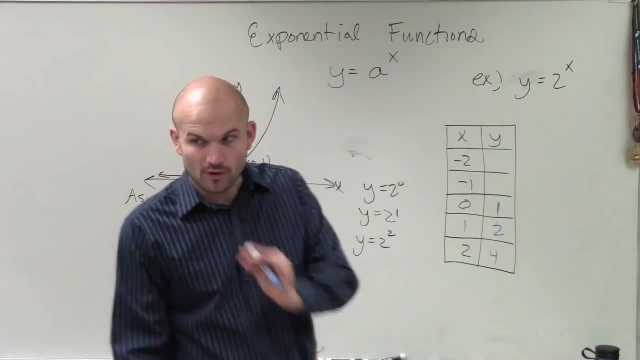 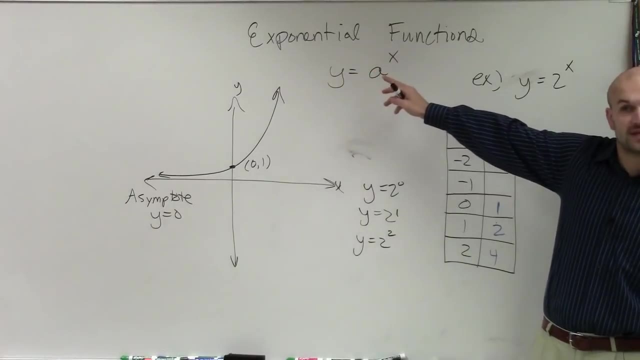 is going to have a y-intercept at 0, 1.. So that's a very important note. It does not matter what your a is. a can be 99 million. You raise 99 million to the 0 power. it's going to have a y-intercept at 1,. 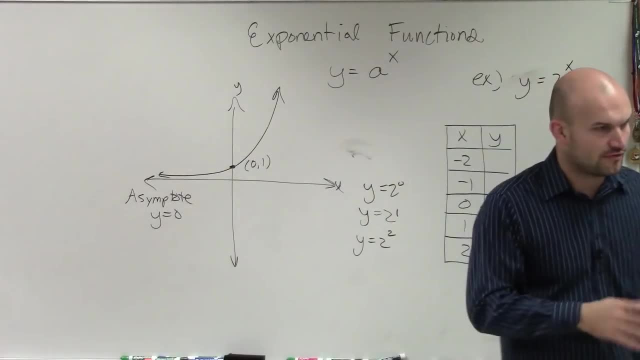 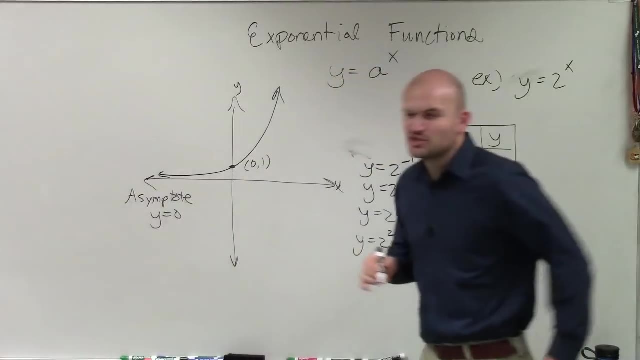 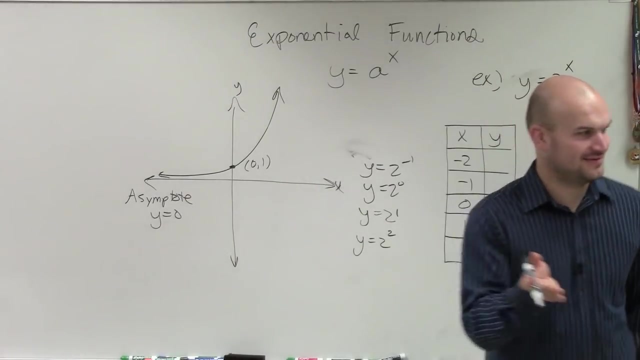 unless you are transforming the function in some form, which we'll get into next. Now we get to the fun ones. y equals 2 to the negative 1.. Anybody remember? I got one answer for negative 2.. I got one answer for 1 half. 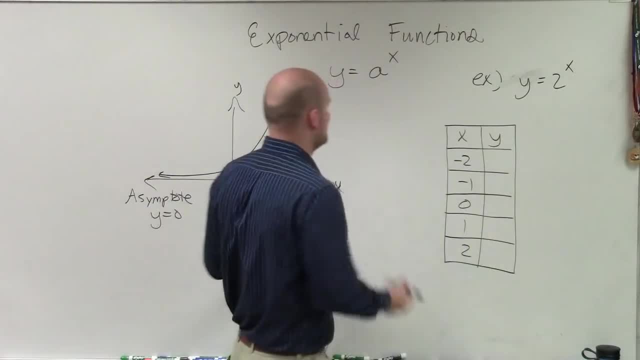 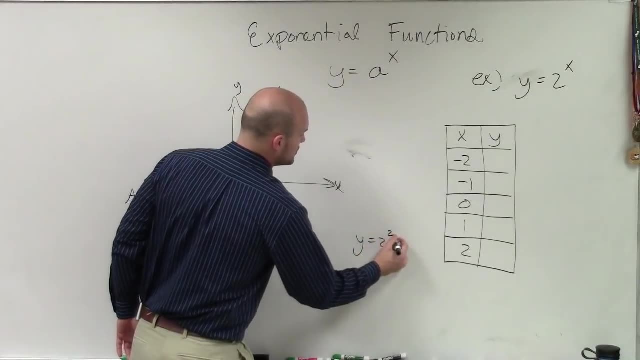 Plug them in. then you find the value of y right. OK, So let's start with the positive so we can remember what it looks like. So I'd have: y equals 2 squared. Well, we know, 2 squared, right. 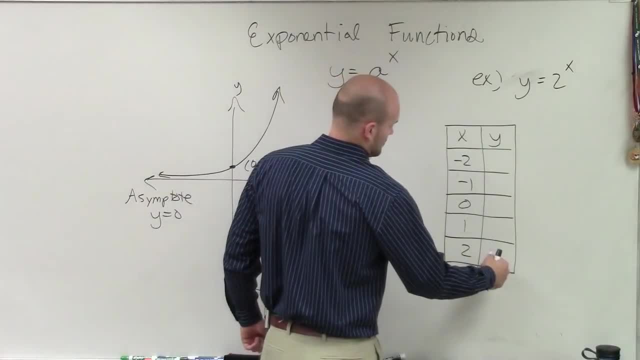 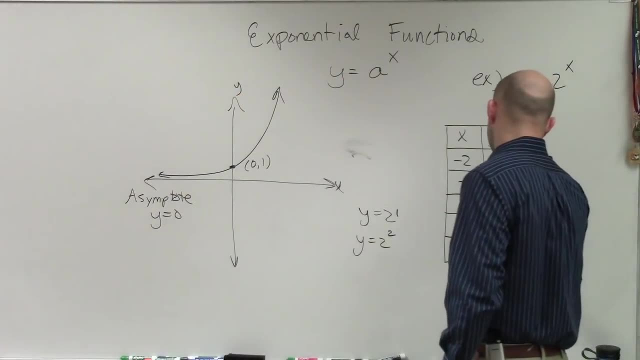 That's 4.. So I'd have y equals 2 squared. Well, we know, 2 squared, right, That's 4.. Y equals 2 to the first power, 2.. So then we have y equals 2 to the 0 power. 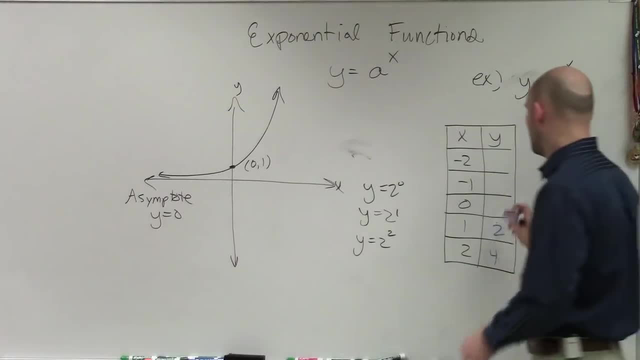 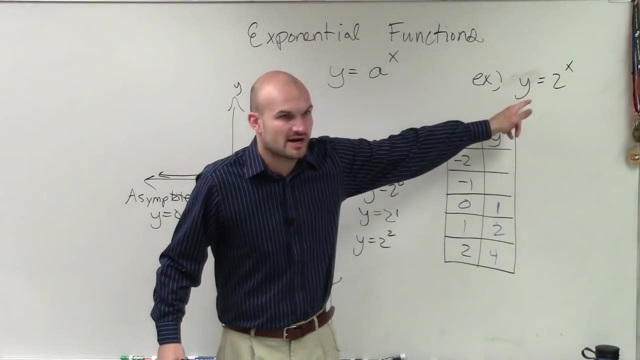 1.. Very good, That's always going to be 1, right, And what I want you guys to understand. some of you might say: well, what happens if my base is 10?? Because we're going to use a lot of different bases, right. 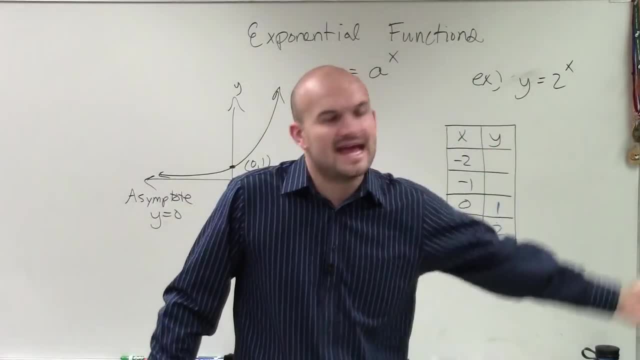 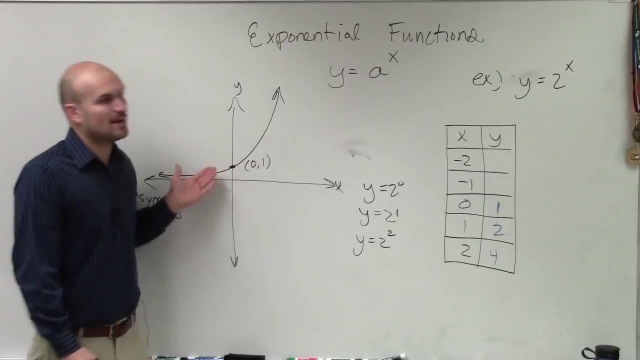 What happens if my base is 10?? What happens if my base is 8?? What happens if my base is 1 half? How is that going to change the graph? Well, one thing: it is going to affect how the graph increases where it's at. 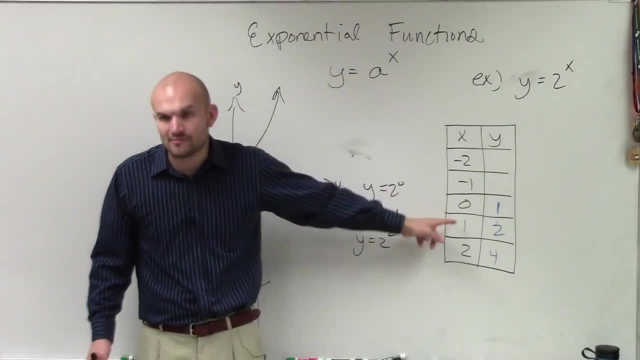 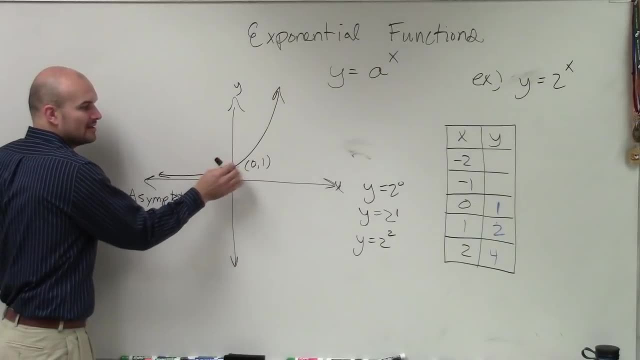 But you guys notice, does it matter what the base is when I raise it to the 0 power? No, So all of my exponential graphs, unless we have a transformation, is going to have a y-intercept at 0, 1.. 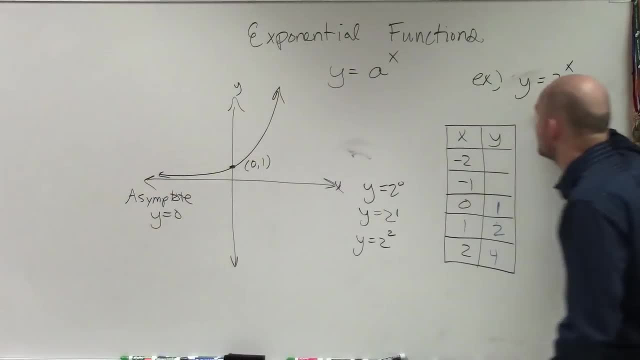 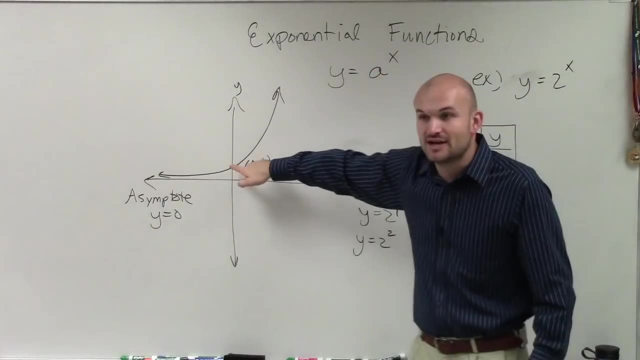 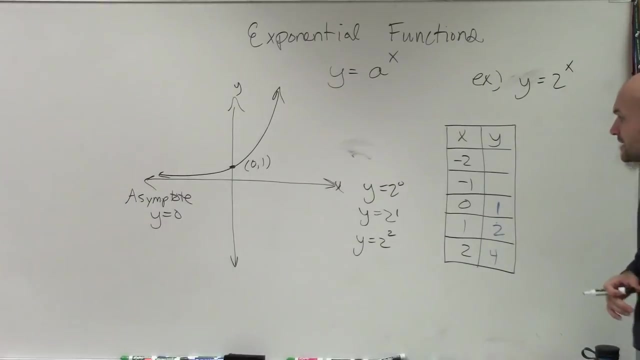 So that's a very important note. It does not matter what your a is. a can be 99 million. You raise 99 million to the 0 power, it's going to have a y-intercept at 1. Unless you are transforming the function in some form, which we'll get into next. 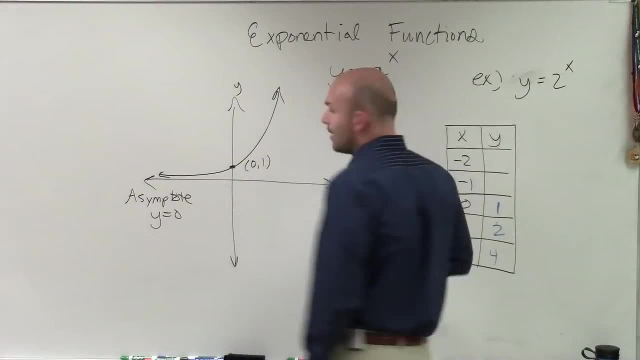 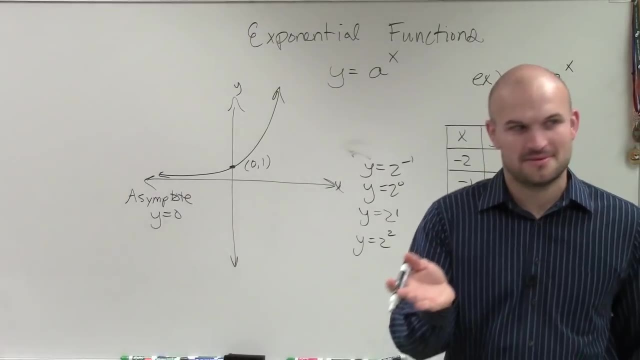 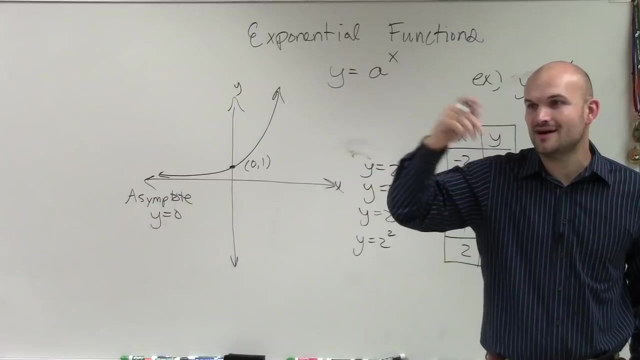 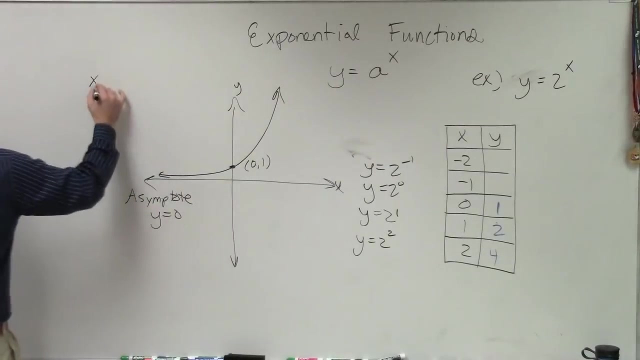 Now we get to the fun ones. y equals 2 to the negative 1.. Anybody remember I got one answer for negative 2.. I got one answer for 1 half. A couple of things we need to remember about exponents. 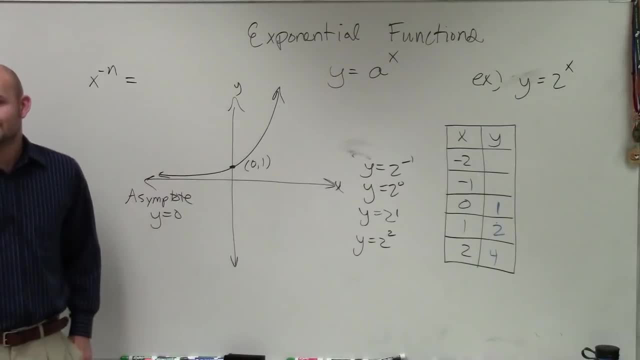 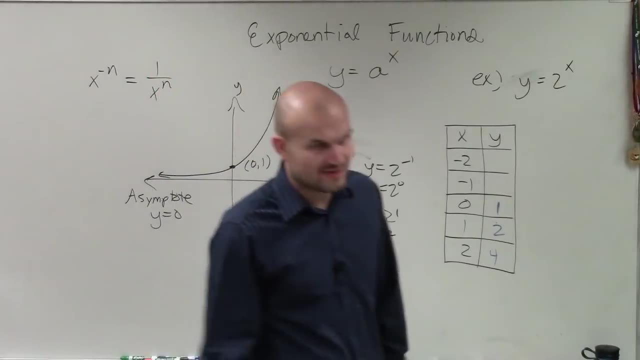 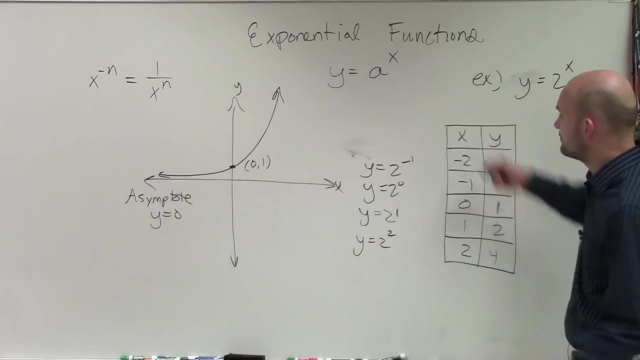 x to the negative, n is equal to 1 over x to the n. That's our properties of exponents. We just need to come back with like, oh yeah, okay, okay. So negative 2 is a very common thing. But remember, all the negative exponent tells you is that this is now going to be y equals. 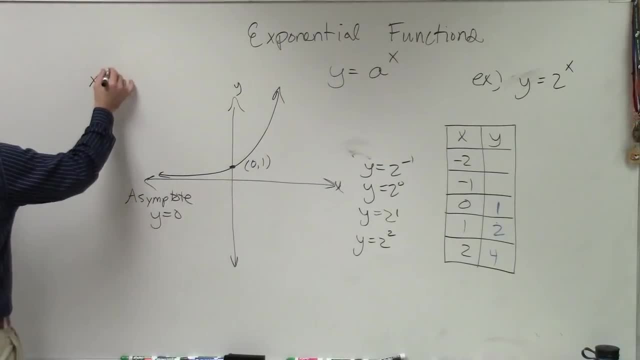 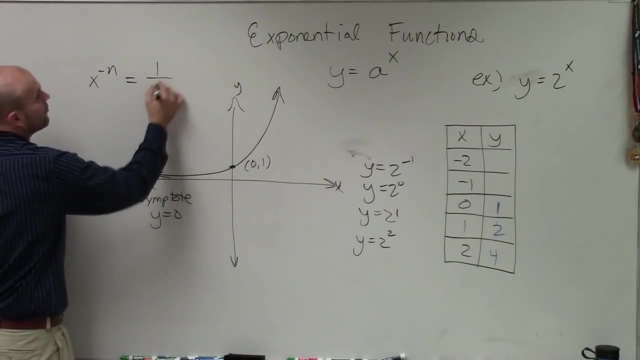 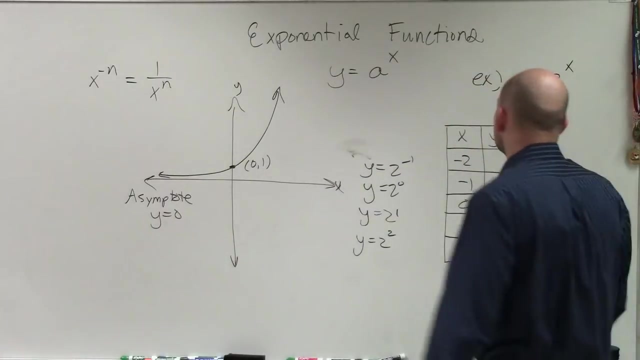 Couple things you need to remember about exponents: x to the negative, n is equal to 1 over x to the n. That's our properties of exponents. We just need to come back with that. So negative 2 is a very common thing. 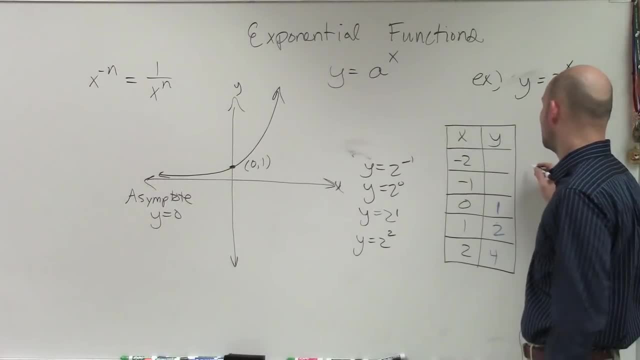 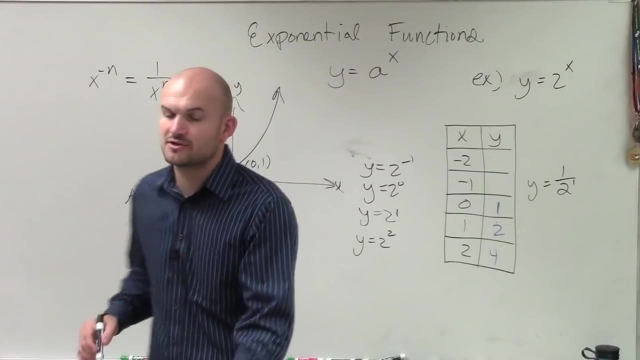 But remember, all the negative exponent tells you is that this is now going to be: y equals 1 over 2 to the 1 first power, And 2 to the first power is going to be 1 half, 1 half. 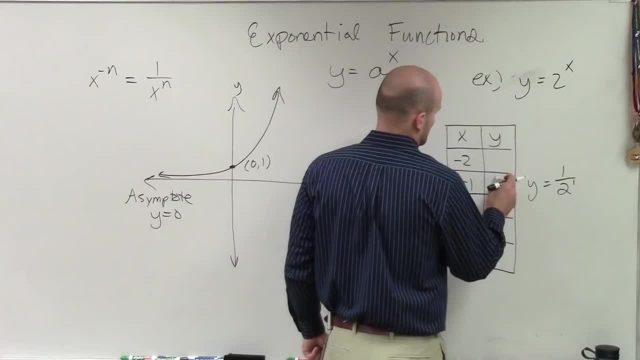 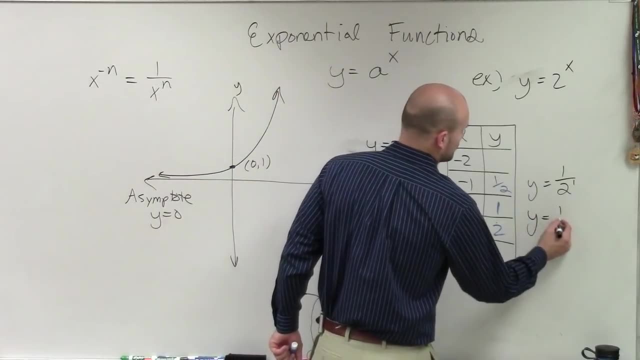 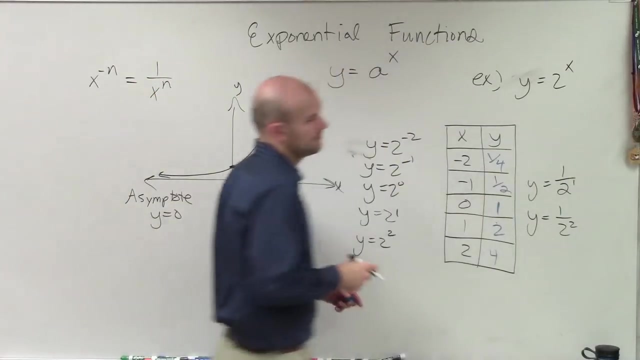 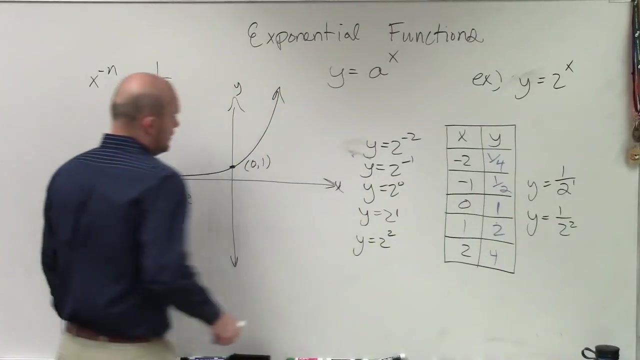 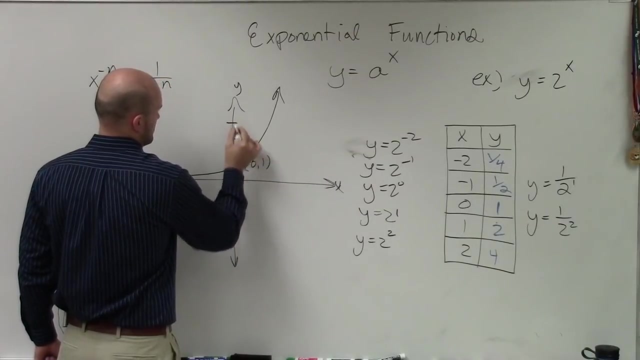 So therefore, y to the negative. second power is going to be: y equals 1 over 2 squared, which is 1 fourth. So now, ladies and gentlemen, let's go ahead and graph this, If you guys look, let's do it at negative 2.. 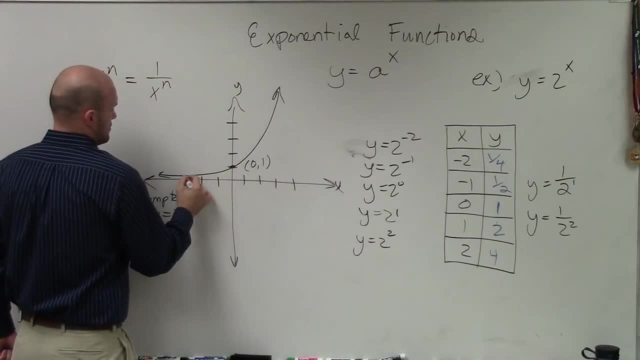 At negative 2, I'm at 1, fourth At negative 1, I'm at 1, half At 0, I'm at 1.. At 1, I'm at 2. And at 2, I'm at 4.. 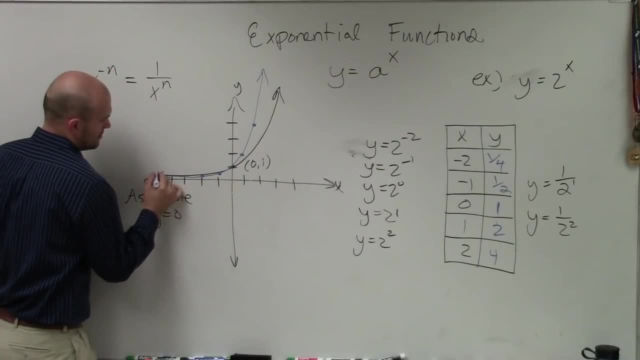 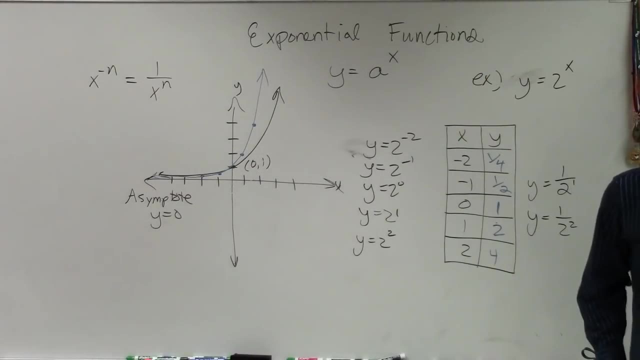 So what's the answer? It's negative, 1 over 2 squared, which is 1 over 2 squared, And therefore you can see what the graph would look like- Very similar to that graph in the black that I drew, But this one looks like it's going to have a little bit. 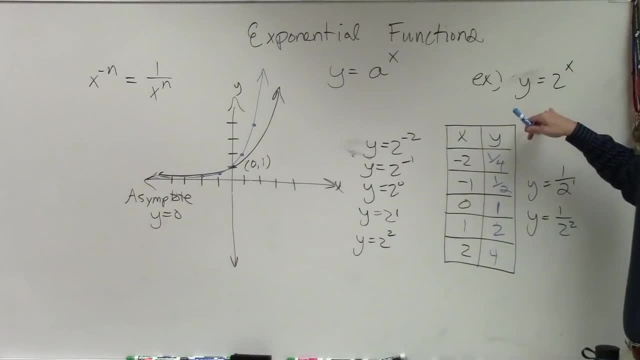 steeper incline. And guess what, If I change this to a larger number, that would probably even have a greater one as well. right Yeah, Maybe. And the fractions are even going to be more interesting. We'll talk about those later. 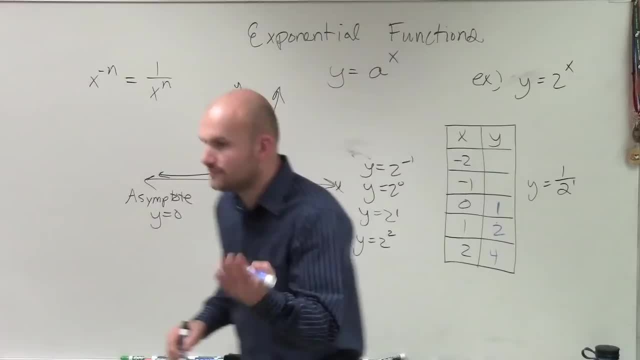 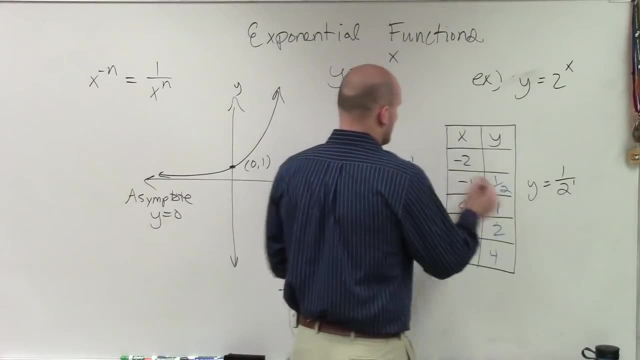 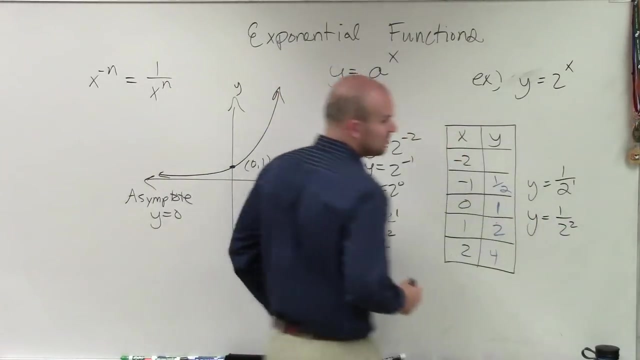 1 over 2 to the 1. And 2 to the first, power is going to be 1 half. So therefore y to the negative. second power is going to be: y equals 1 over 2 squared, which is 1. fourth, 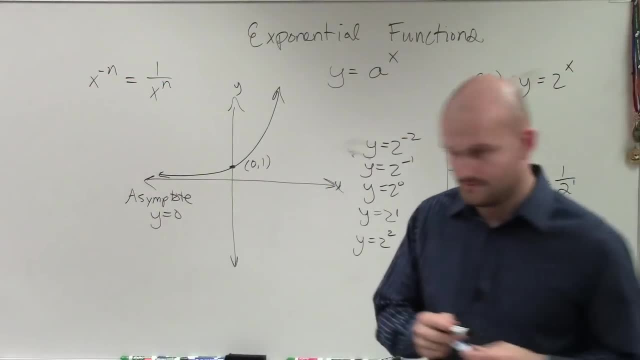 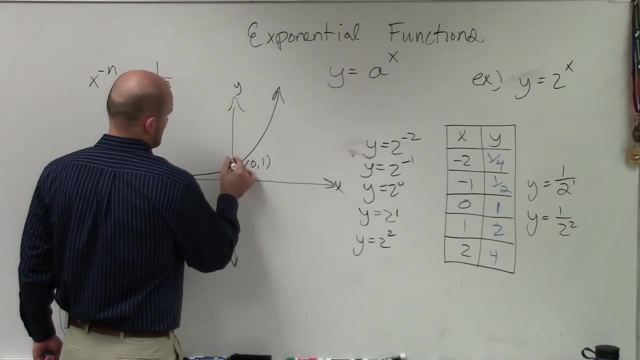 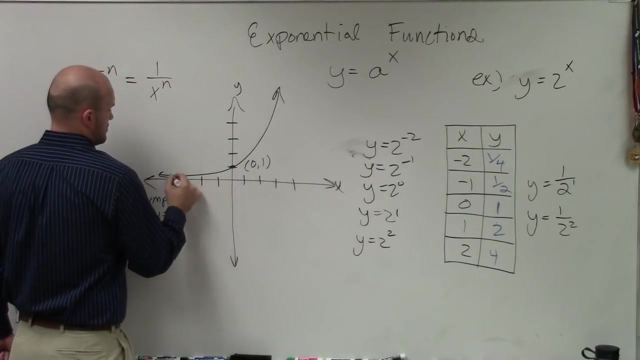 All right. So now, ladies and gentlemen, let's go ahead and graph this. So, if you guys look, let's do it at negative 2.. At negative 2, I'm at 1 fourth. At negative 1, I'm at 1 half. 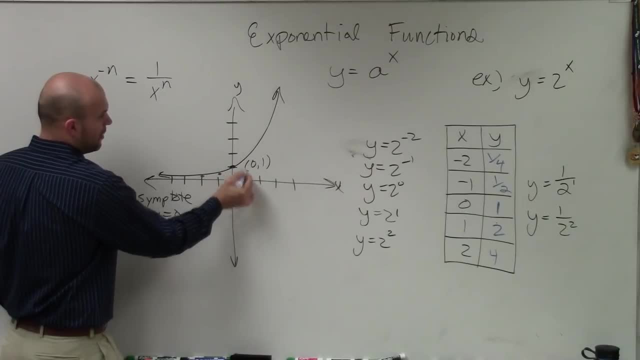 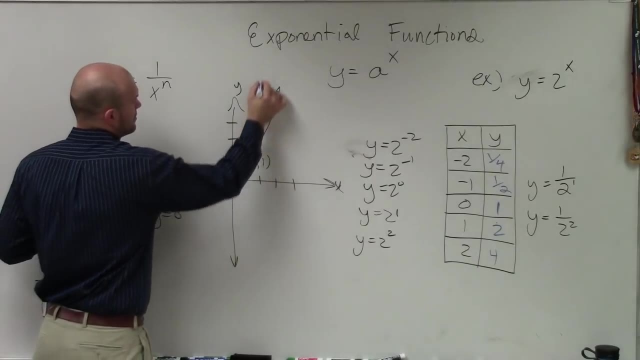 At 0,. I'm at 1.. At 1, I'm at 2. And at 2, I'm at 4. And at 2, I'm at 4. And at 2, I'm at 4.. 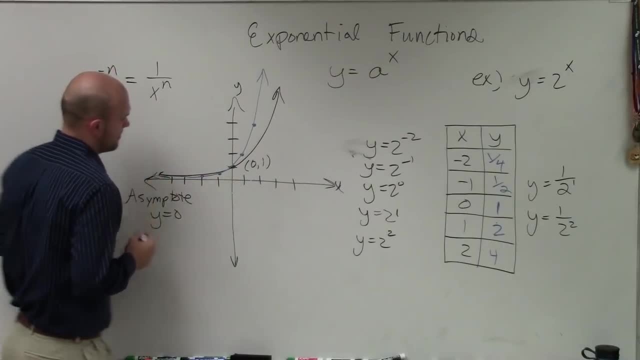 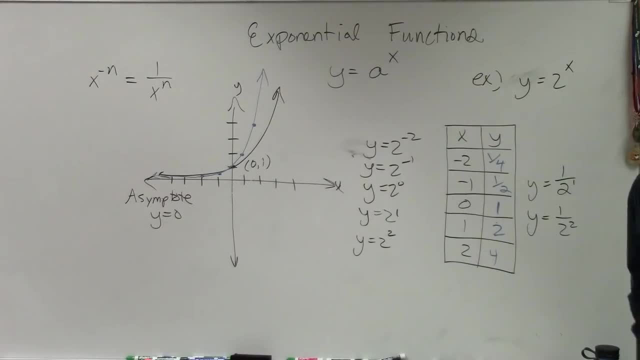 And therefore you can see what the graph will look like. All right, Very similar to that graph in the black that I drew, But this one looks like it's going to have a little bit steeper incline, right, And guess what.